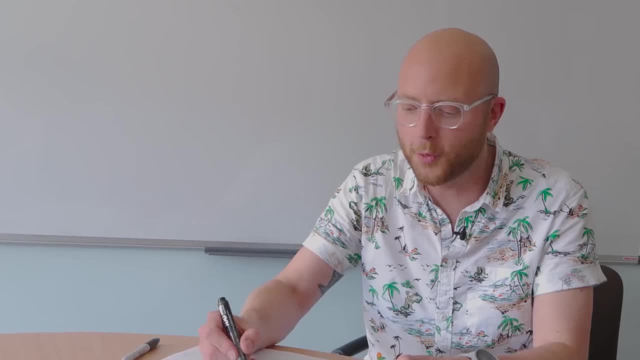 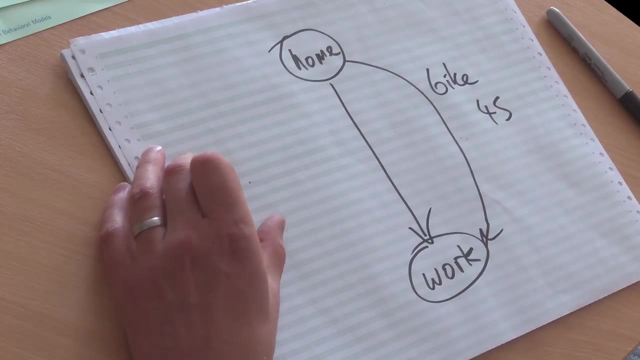 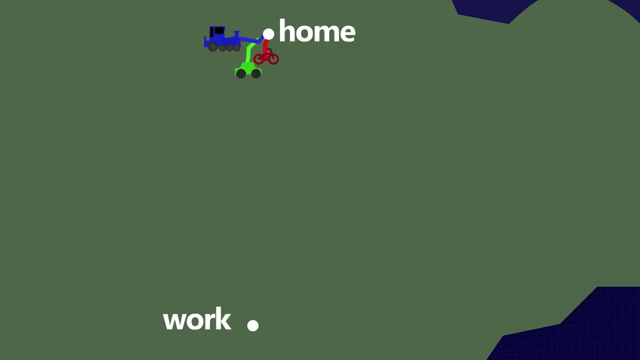 for that later. But you've got, let's say, the simplest, shortest path problem. You've only got one action. so you can go by bike, and that might take you 45 minutes. And you can go by car, and that might take you, let's say, 30 minutes. And you can go by train, and maybe that takes you 35.. 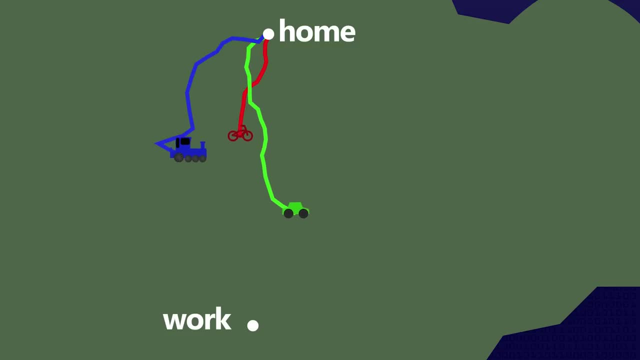 This is a kind of a standard decision making problem. right, We've got two states, So our states are being at home or being at work, And we've got three actions, So we can go by bike, we can go by car or we can. 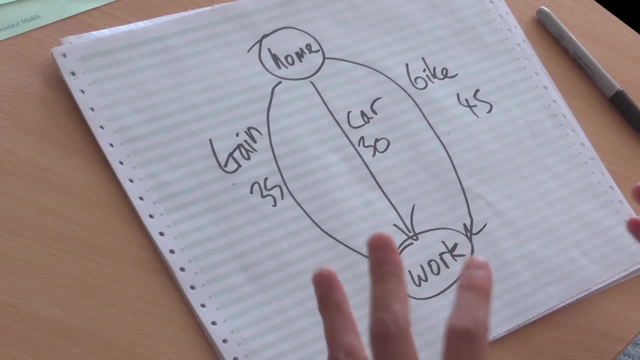 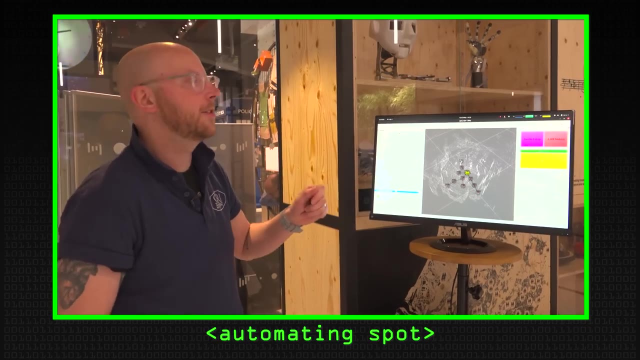 go by train. We use these kind of state transition models everywhere for robotics. So if I'm programming a robot to pick something up or navigate between in a map- Last time we were together- we're looking at robots navigating through these graphs and we turn those graphs. 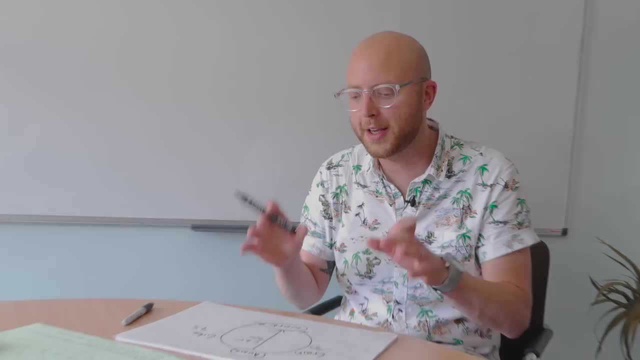 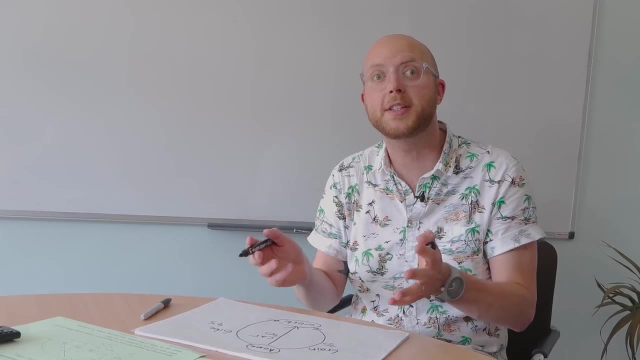 into these kind of decision problems as well. So this is a kind of a model you could use to decide: well, what route do I use to get to work? And in this case, if we're trying to minimise time or minimise cost, then we would take the car option, which is 30.. I'm going to do my teacher thing. 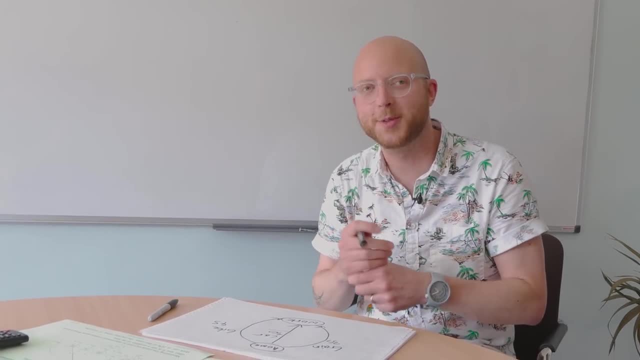 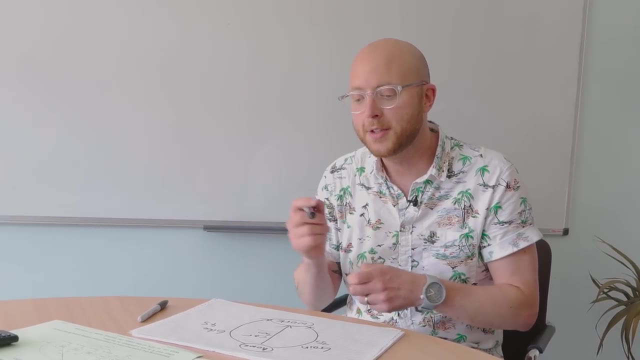 What's the problem with this model? It's too simple, right, It's too simple, So it doesn't reflect the fact that life is just. yeah, the world can be against you, So the world can be uncertain. So the standard thing we do in robotics is we take 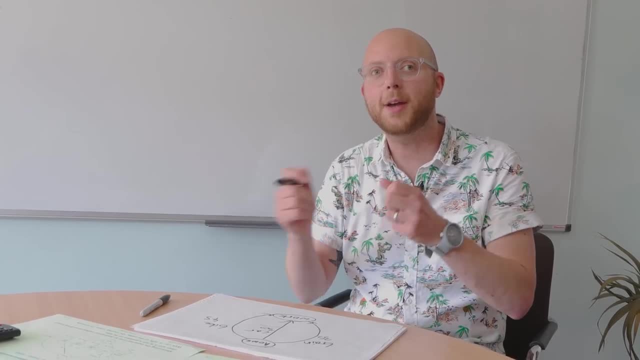 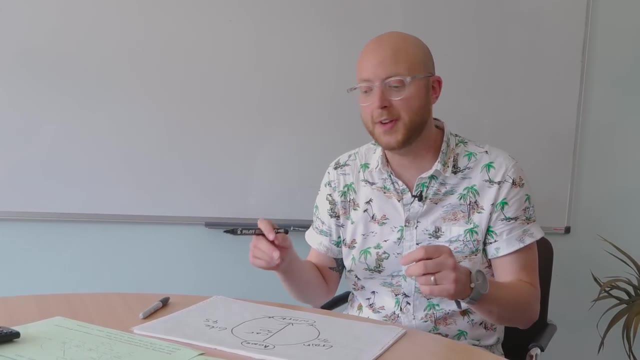 these what we call deterministic models. So this is a model where the outcome is fully determined by the state You're in, so you know where you're going to be And we can say: well, we can. actually, we can- make them more complicated. We want to reflect the uncertainty, So I'll draw a kind of a big version. 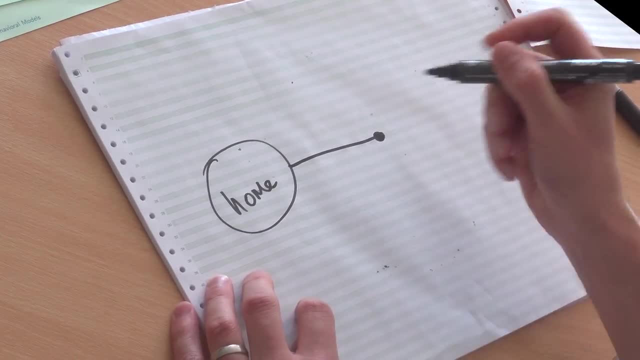 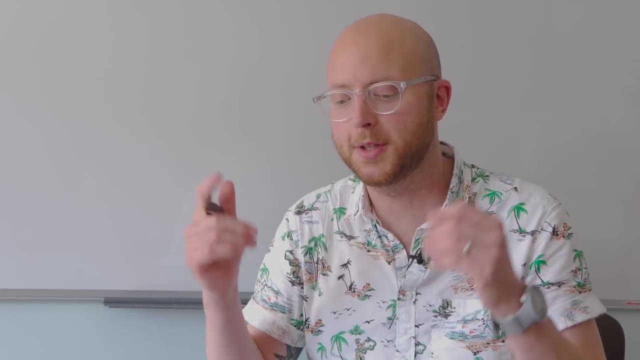 first and we can think about that. So we imagine we take our action, which we might call car, and that's still going to cost us 30, or it's going to take 30 minutes. right, That's my planning model. This is how we're going to model the world. But then what we're going to think about is actually: 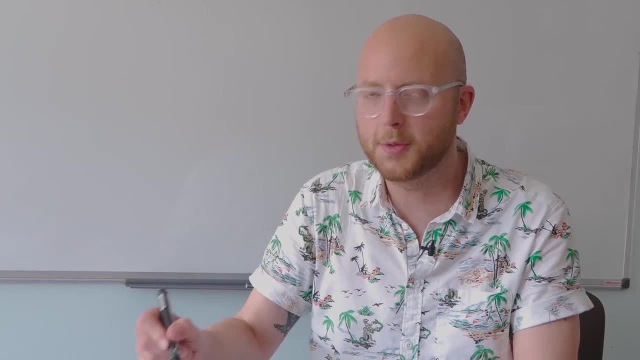 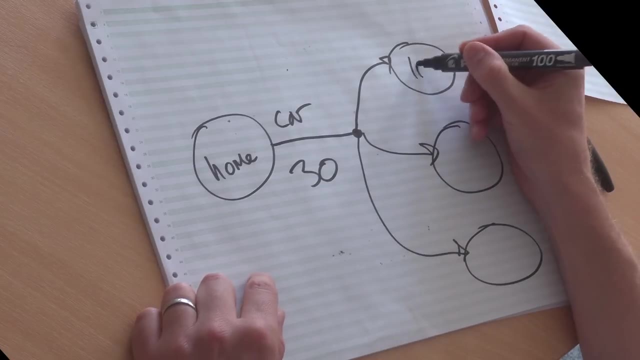 there are going to be different outcomes. So when I execute this action, so when I perform that action in the world, I can still only end up in one of three different states. but they might be different traffic levels, So it might be light, medium and heavy. That's kind of imagine. I've got in my car, I've chosen to take my car to work. 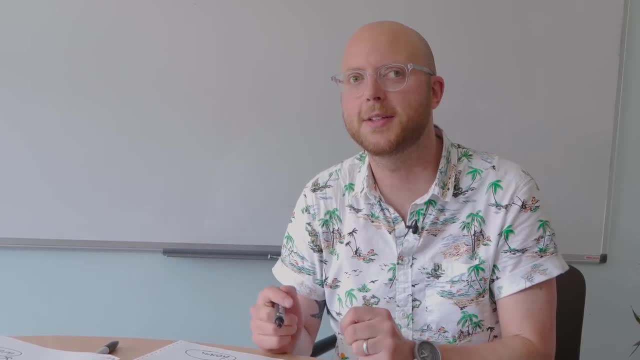 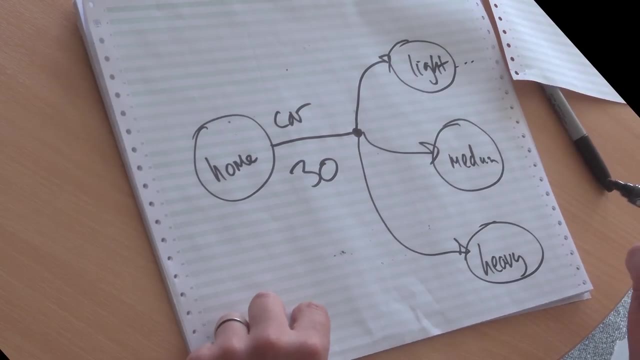 I've driven a little way and I hit the motorway or whatever, and it's one of these traffic states, and then I can go to work from that. But what we could imagine is when we move out of those states, it's going to take us a different amount of time. So what we might do is we might use that to change. 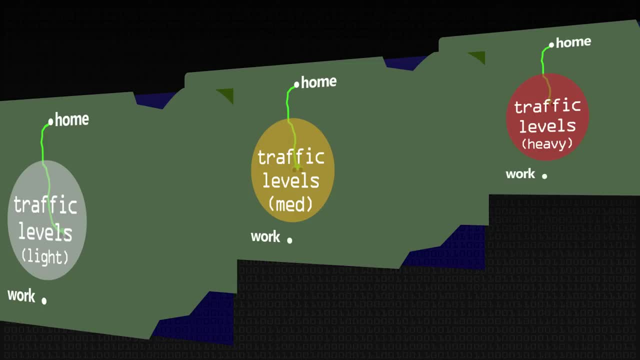 our model. So this is the basic idea, and what we would do is we'd assign different probabilities. We might say 20 percent of the time, or 0.2 the traffic's light, 70 percent of the time it's medium, 10 percent of the time, or probability of 0.1 there's heavy traffic. So this is reflecting. 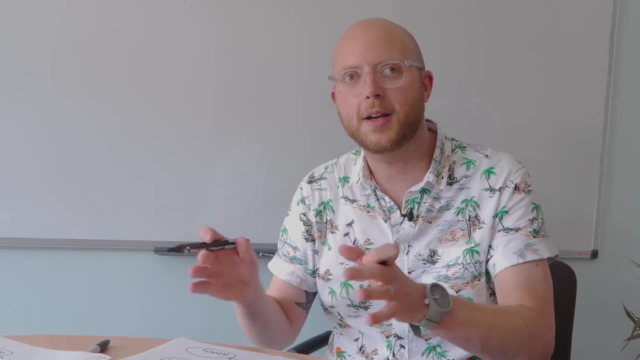 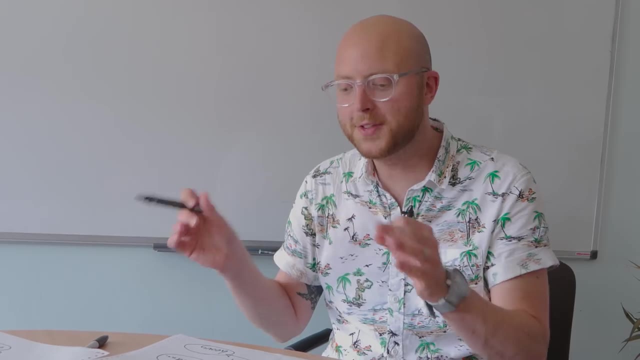 some of that uncertainty, some of that complexity in the world. This is kind of the standard action model we'd use, and when we use action models like this, this is called a Markov decision process. So a Markov decision process is states and actions just like a shortest path problem. 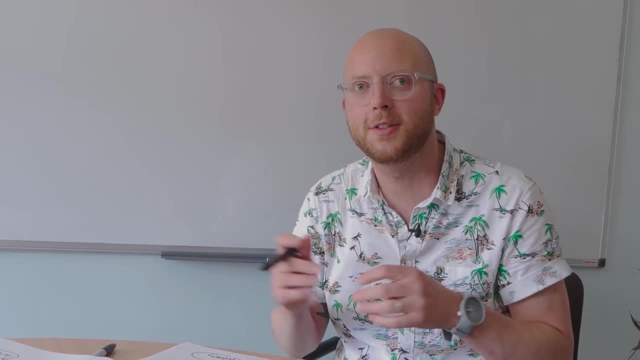 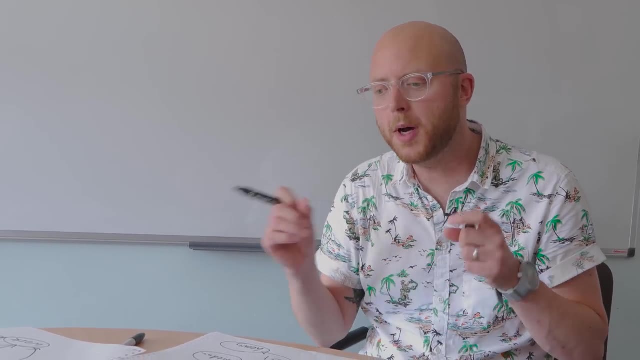 except now, when I take my action, there's a probability distribution over the the outcomes I can reach. I think Markov sometimes talks about the tax, isn't it? is that right? Yeah, so Markov is a probabilistic assumption. when you've got a state, it doesn't need actions, right? 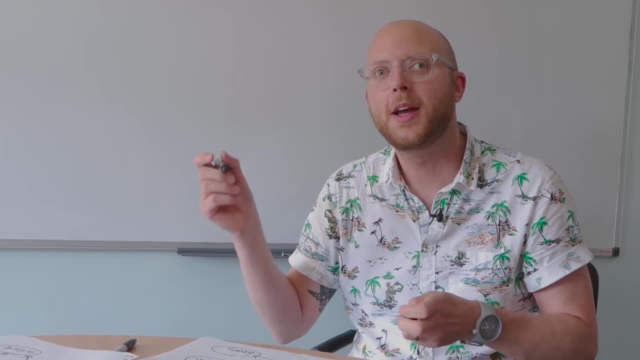 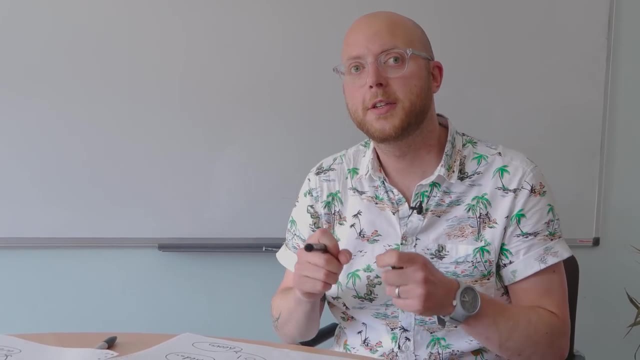 it can just be state transitions, excuse me, state transition systems. and what we do is a Markov assumption says the probability of an outcome only depends on the current state. So it doesn't matter the history, it doesn't matter what I was doing before I chose to leave home. the only thing 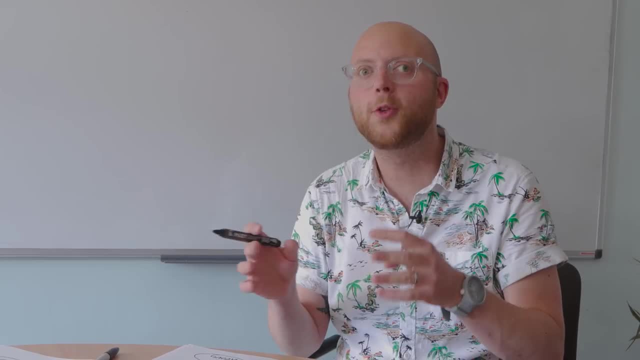 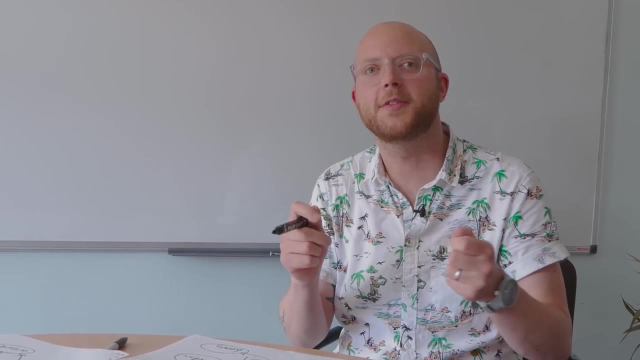 that determines that probability is the action I'm taking right now. To be more formal, you can think of that as a sort of first order Markov system and you can have a second order Markov system which says only the current state and the previous state determine my probabilities. But in general, if you 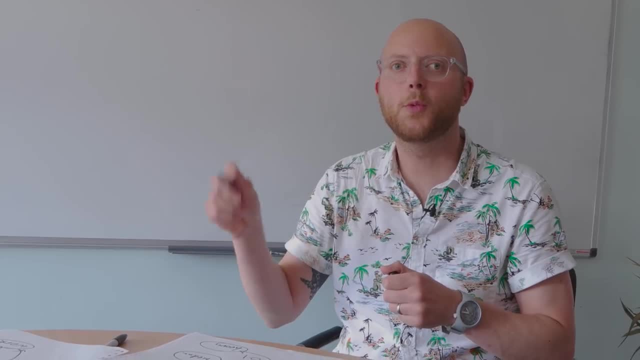 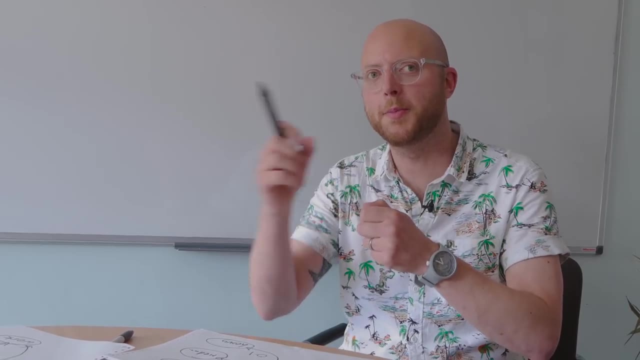 think of something like a Markov chain. if you're doing text processing, you can think about word generation following probability distributions, and there you can think of like one step: so if I give you the, there's a probability of getting cat. or if you, if I give you, I am the, then you get a. 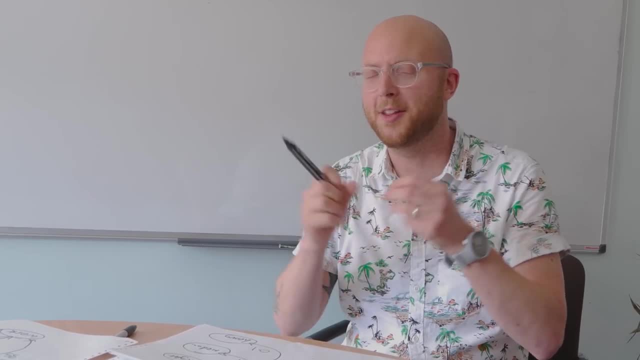 probability of getting something different. and if you take that whole history so you make- I think that would be a third order Markov assumption. So you can think of that as a probability of getting cat, You'd get a different probability distribution over the word you'd get next. 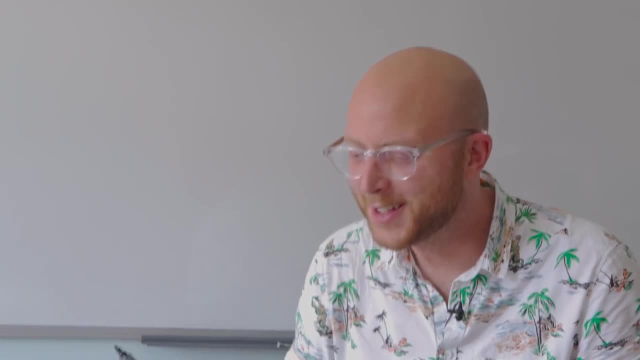 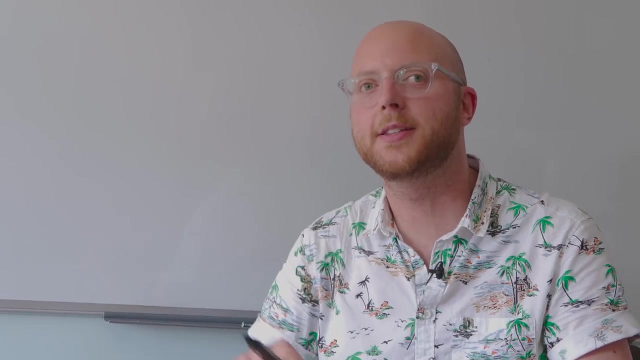 I'm desperate to say: walrus Cuckoo ca-choo, Right, so that's our kind of action, that's our action model, and so we can take this action model, we can stick it into the, the graph we had before, the process we had before. 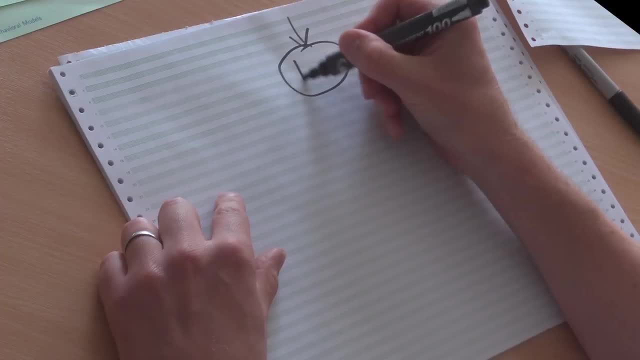 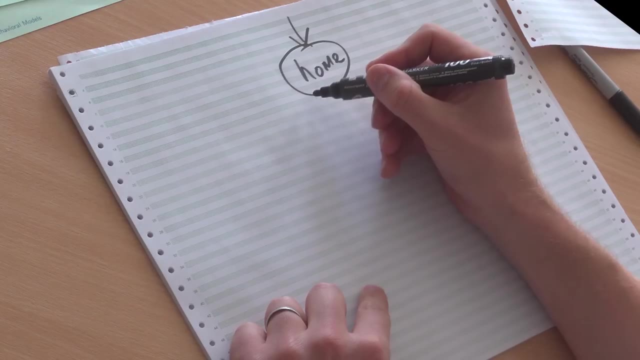 Let's set this up again and we'll draw that little arrow at the top. that means this is our initial state. so, just like a shortest path problem, we're going to start from somewhere, and we typically do this in robotics, because our robot has to be somewhere when it starts thinking. 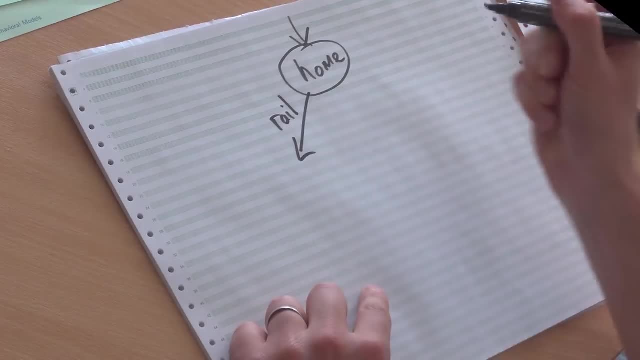 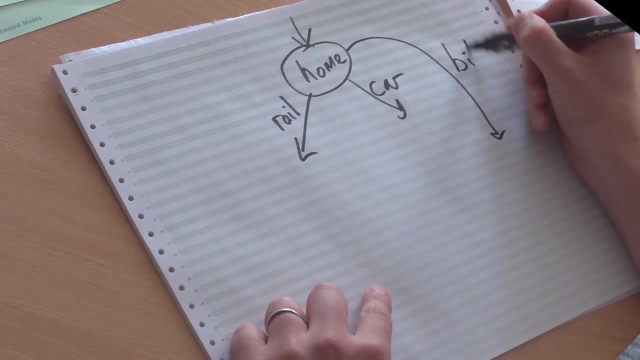 So we're going to make our whole world a bit more complex. so I can either go to the railway, I can go by car, I can go by bike. so these these actions now really are reflecting the choices I'm going to make to start with. so not necessarily getting on and doing that, but sort of making 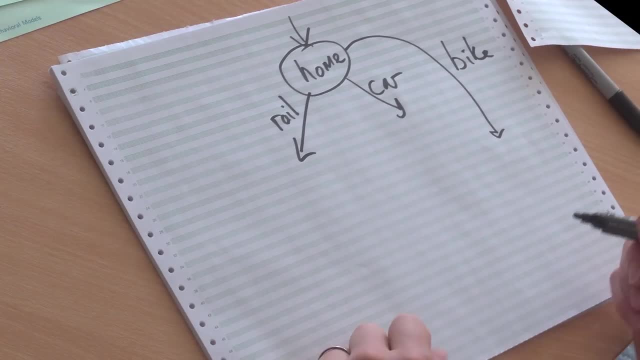 the decision that this is what I want to do and maybe go into that form of transport. so now car is going to take one. this is me leaving the house and going to my parking space and finding my car- railway. maybe I have to walk a bit further to get to the railway, so that'll be a cost of two. and then 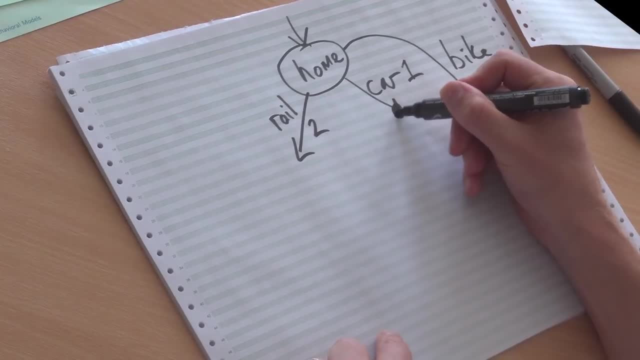 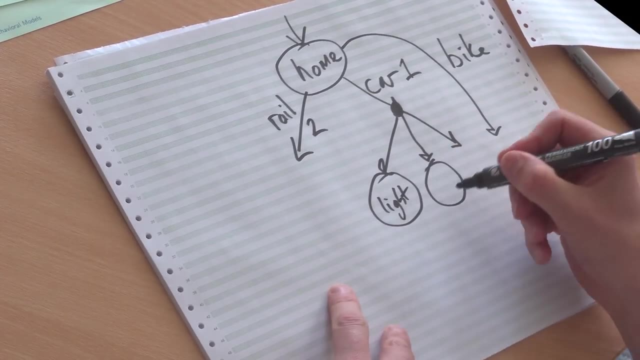 start to put these, these actions in. so actually these arrows should be dots and I can put in the action that we had before where we have different traffic levels, so light we've got medium. I'm going to start abbreviating these things because my handwriting is atrocious and will take forever. 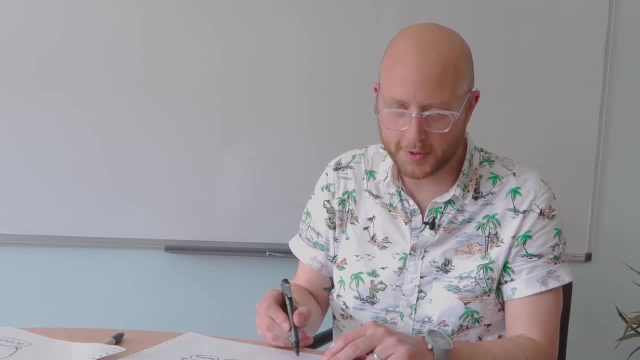 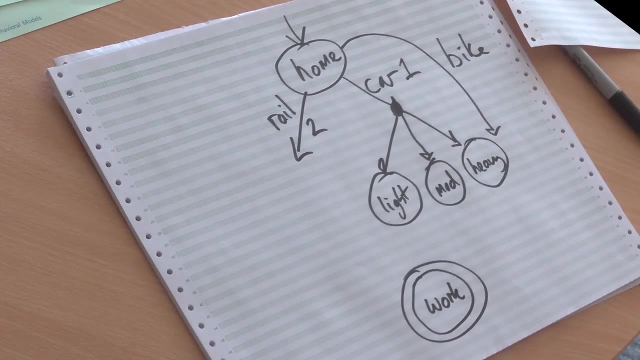 just watching me write words or heavy and then down at the bottom, down here we're going to have work, and I'm purposely doing two circles here because we've got this state transition system. we have our initial state with the arrow coming in, and I do these two rings to mean this is where we 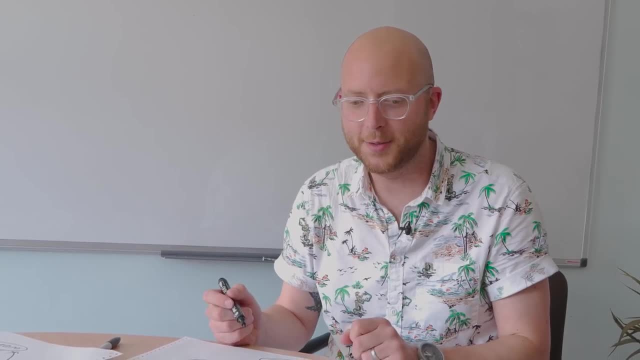 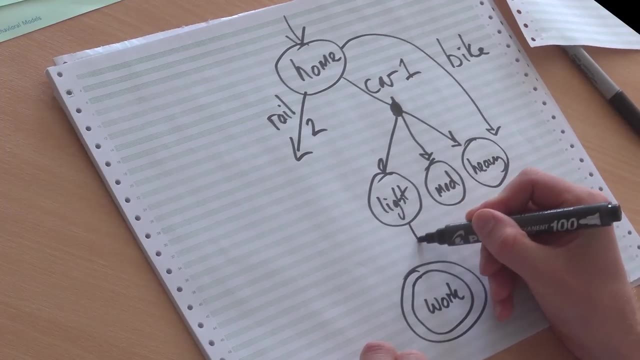 are going to go and then we have our action called drive. so there's no, there's no way to get out of it. when you're there and, as this is work, that's a little bit depressing, but there we go and then we might have an action called drive. so our drive action is going to be deterministic. 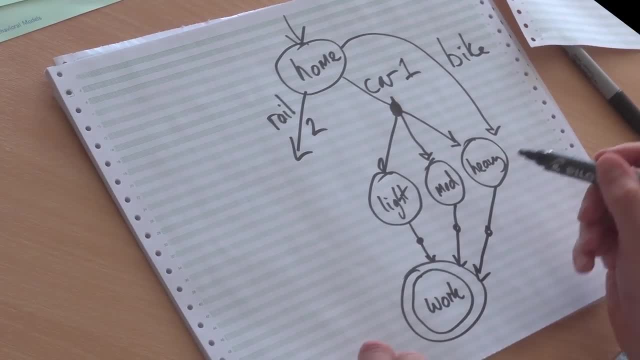 in that I can take it, and it always takes me to work, but I can only take it in certain states. so I can only take it once I'm in my car. I'm only allowed to drive then, and we can use this now to model the fact that we might get different durations of travel. 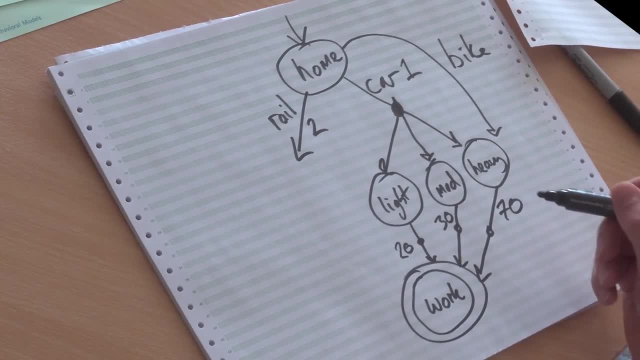 so in heavy traffic it takes me 70 minutes to get to work. in heavy traffic, 30 and medium, 20 minutes in light, and I think we had these probabilities of 0.2, 0.7 and 0.1. so this shows me that if I go by, 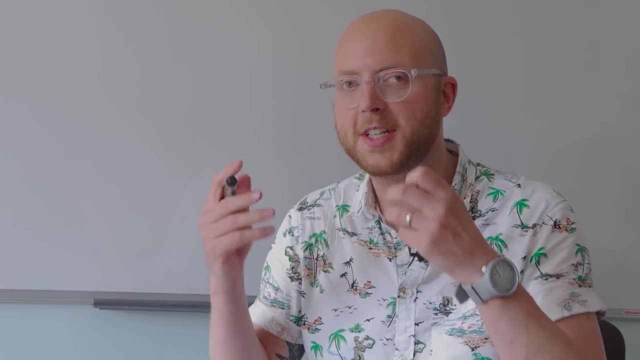 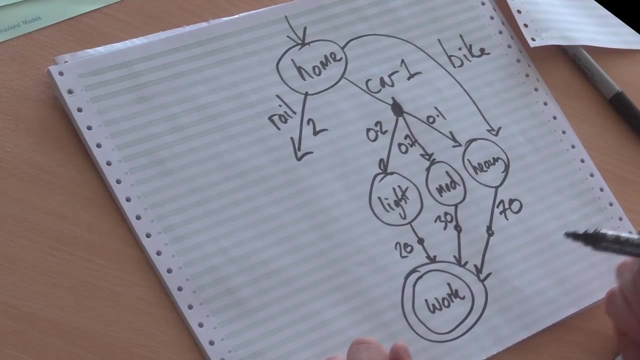 car I get some probability of these different traffic levels and once I've experienced that traffic level there's no turning back. I have to follow the car. I have to follow that action choice. so use the car to get to work and it might take a different amount of time. we're going to say 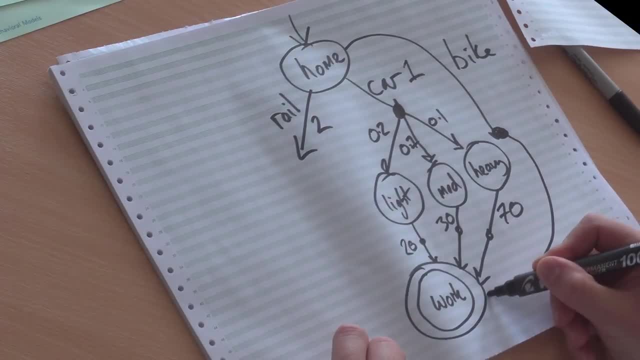 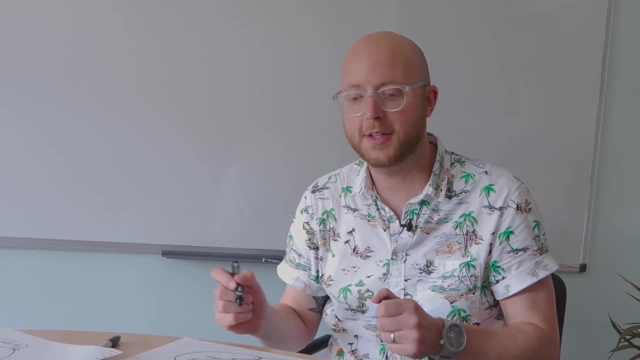 here the bike is deterministic, so if I'm on a bike I'm fully in control of the duration it takes me. so that will take 45 minutes. so it's further by bike. but there's no uncertainty and that could be interesting later. in this example we can say that when I go to the railway station 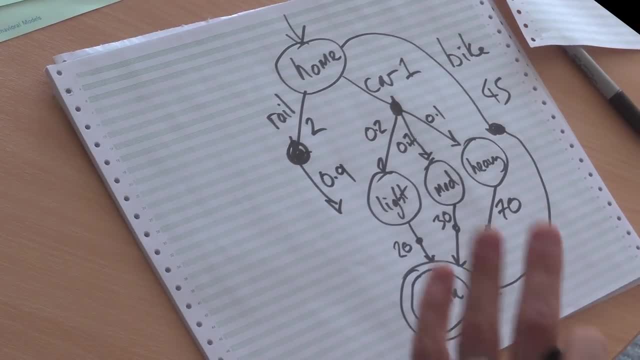 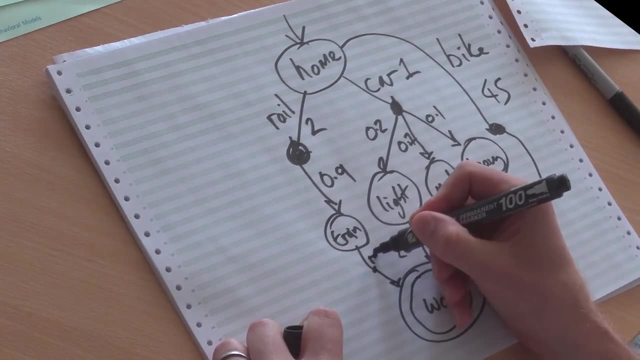 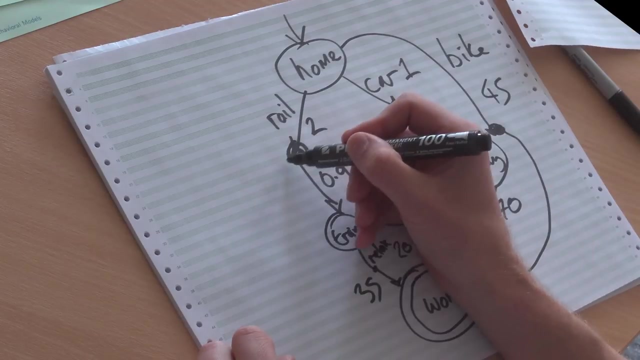 well, maybe 90% of the time it seems quite unlikely. the train is there, it's ready to go, and then it takes me. I've got an action which we'll call relax, because once we're on the train we're happy, and that's going to take me, let's say, 35 to get to work, and then 10% of the time. 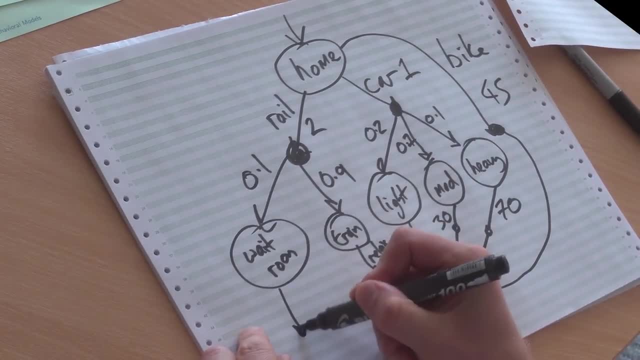 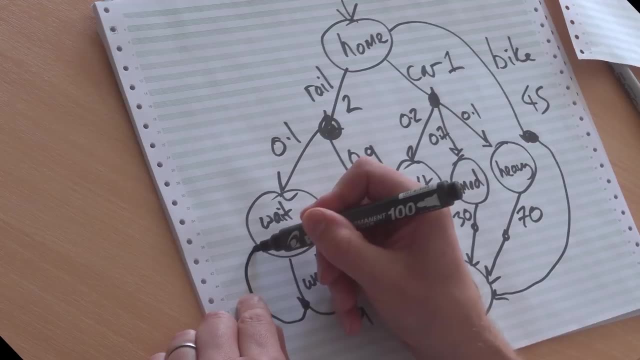 I have to wait. so I'm in the waiting room and then from the waiting room I get to wait, and then 90% of the time the train comes, 10% of the time I get to wait again. so what's interesting here is there's a kind of notion of a time step. you can start to imagine that I'm looping. 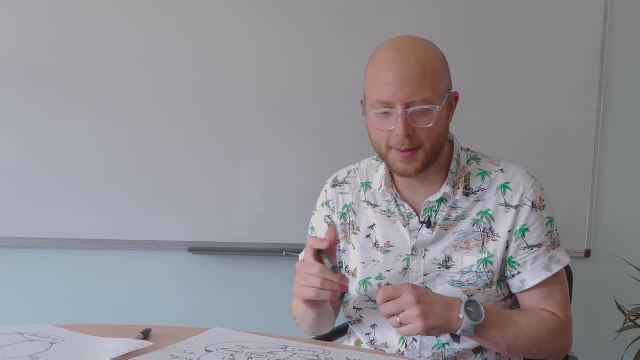 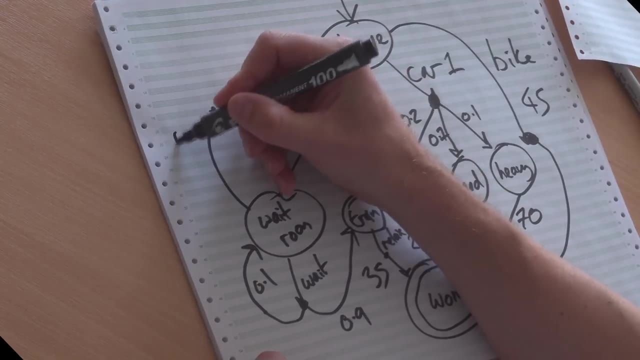 I wait the train comes, I wait the train doesn't come, and I repeat that. and, of course, if I get stuck in the waiting room for too long, I could also choose to go home, and what's nice about that is then I get to make another choice. 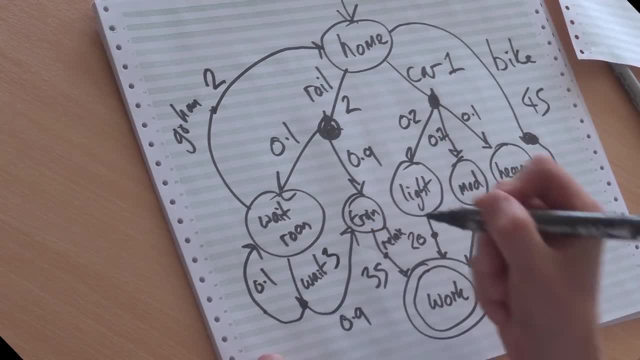 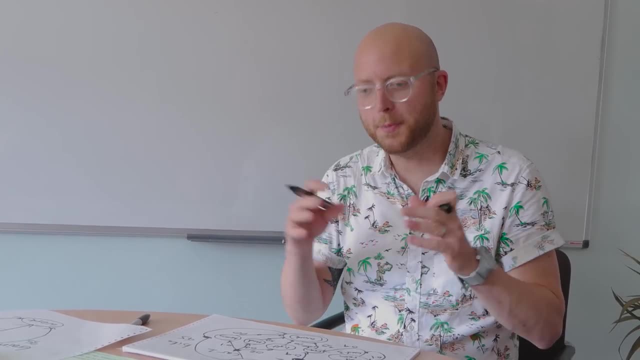 so that might cost me two my waiting. maybe I wait for three minutes each time. so now I've got this big graph and this is the Markov decision process. this is a process because I'm going through a sequence of steps. at each step I have to take a choice over what action. 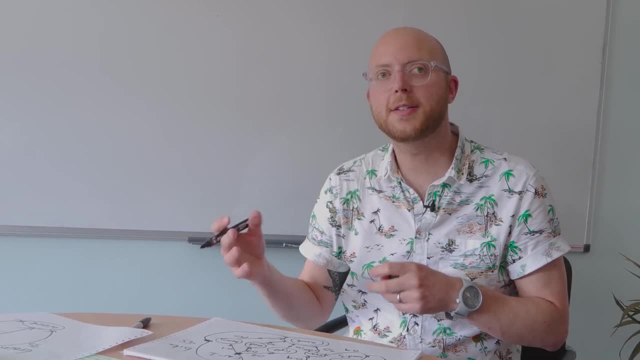 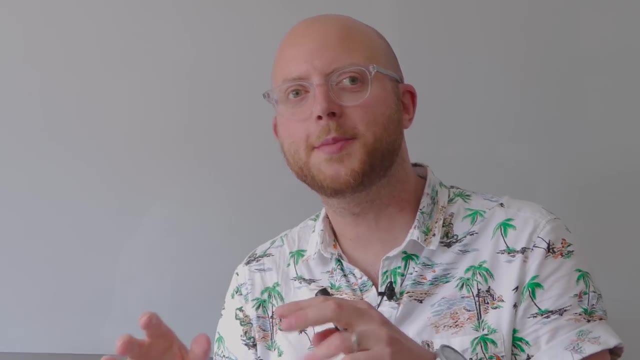 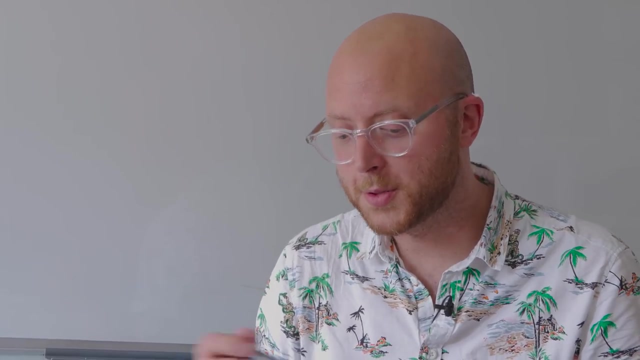 to perform and then that evolves the state. so it changes the state I'm in and we have different probabilities of reaching reaching different states. that's kind of interesting. still, in some sense, we can think about this as a shortest path algorithm, but instead of a shortest path, we call this a stochastic shortest path, because what we want 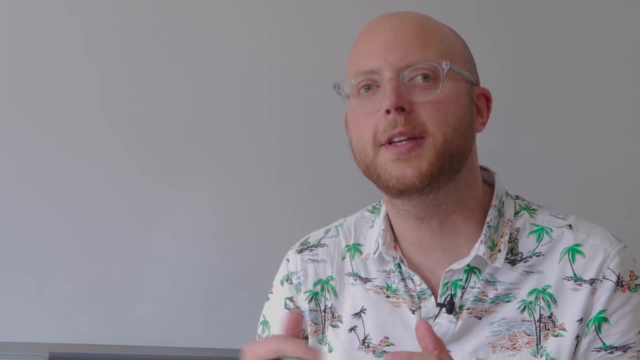 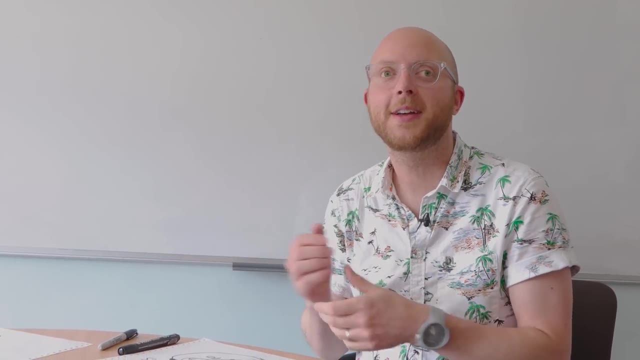 to do is reach our goal. so we're still trying to reach our goal, but now we're dealing with the uncertainty as well. this is a model. this describes the choices your agent could have, so this is the choices you might have when you're going to work. we could imagine I'm building an. 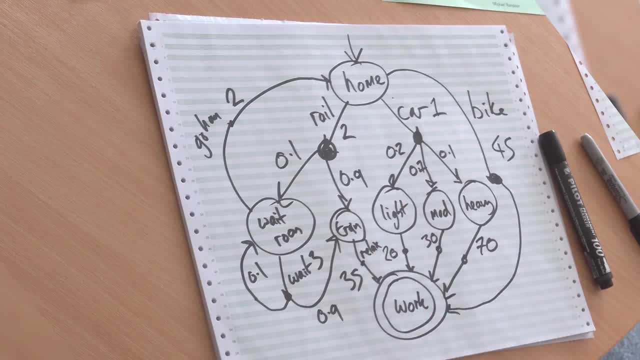 autonomous vehicle and this is, you know, it's an autonomous taxi system and it has to decide how to take you to work. these kind of models really capture what we, the decision. you know a decision-making process can do. you know a decision-making process can do. 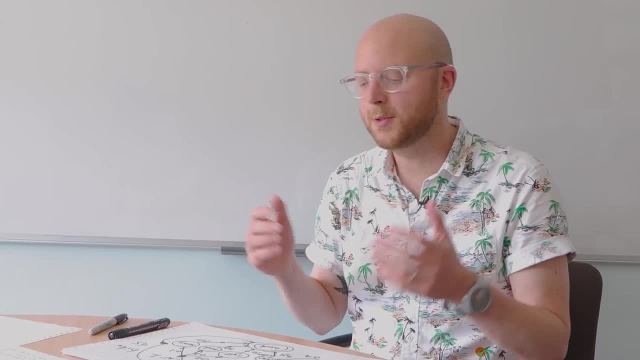 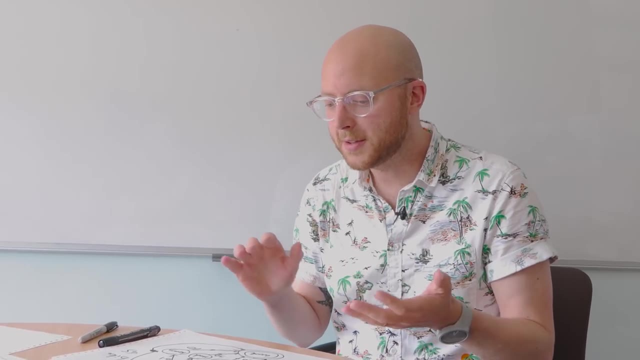 part of artificial intelligence, whether that's robotics, whether that's chat bots, all sorts of stuff, and so the next question is really: how do we, how do we solve this? and there's there's two answers, or there's two parts to that answer. the first thing is: what does the solution look like? 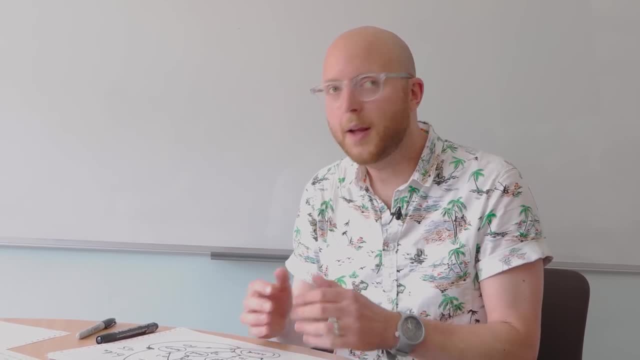 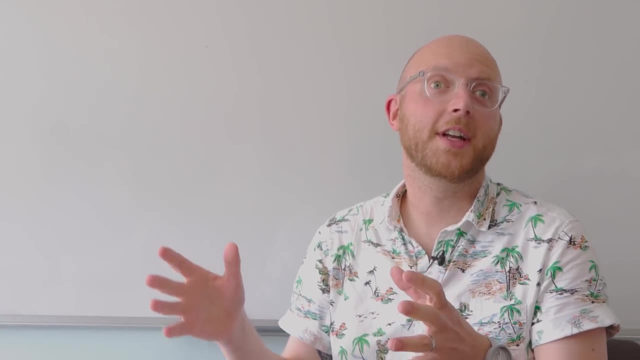 the second bit is: is what? what algorithm do we use when you say: what does it look like? you mean as in? is it? is it just a simple number? or is that what you mean? yeah, well, so in the okay, what structure does the solution have? so, if it was the shortest path problem, the, the solution is a path. 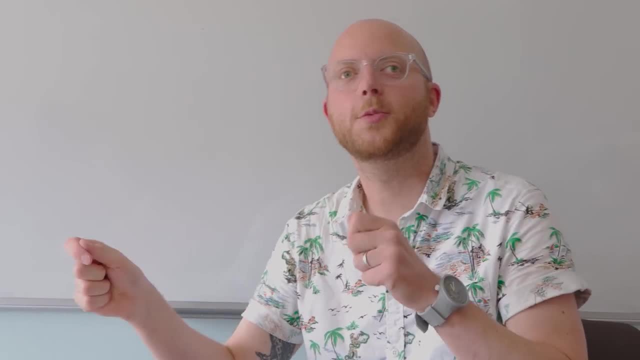 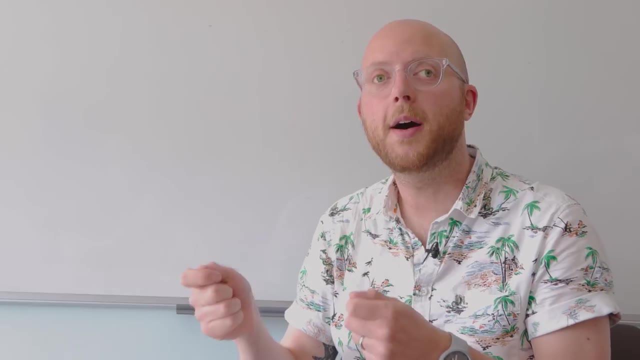 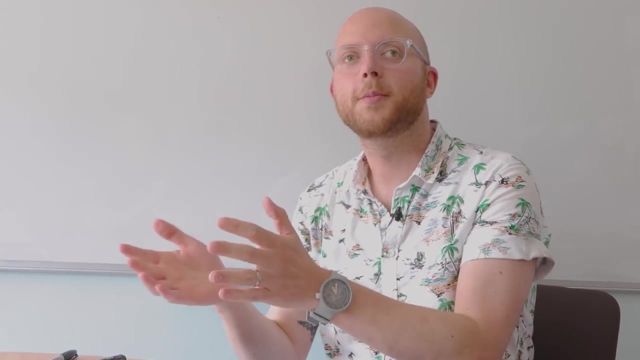 right, it's because it- and that's a sequence of the actions you will take from start to finish. but in in a, in an mdp, in a markup decision process, we can't use a path, because when I take a step, the world changes probabilistically, stochastically, so I I don't know what world I'm, what state I'm going. 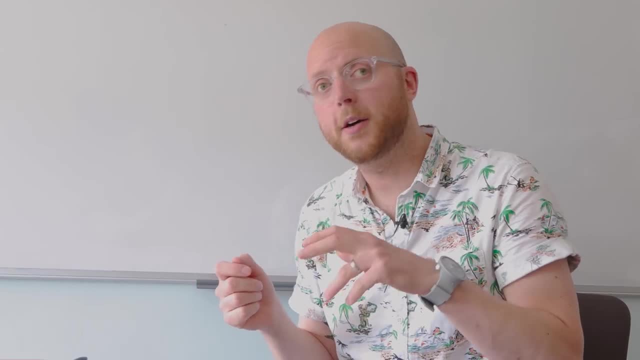 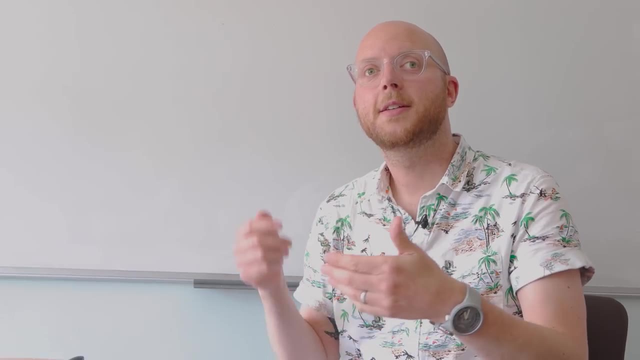 to end up in. so instead of a path, we have what's called a policy. so policy is a lookup table that just says: when you're in this state, take this action, and that state could be the states from the problem, or we could even augment them so as the 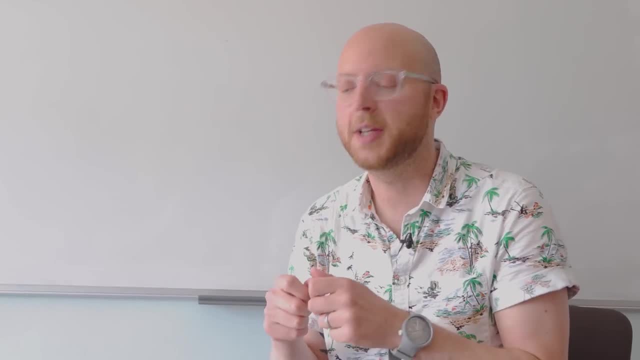 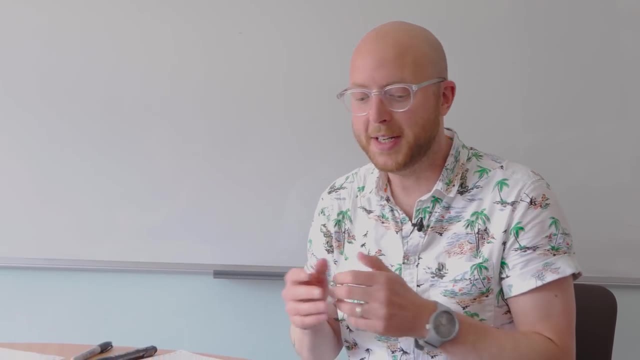 as these models get more complex, we might add extra information into the state. we could add the time of day. we could add: um you know how much time is remaining before some kind of deadline? um, how many times we waited in the waiting room might have been interesting. you can add extra to. 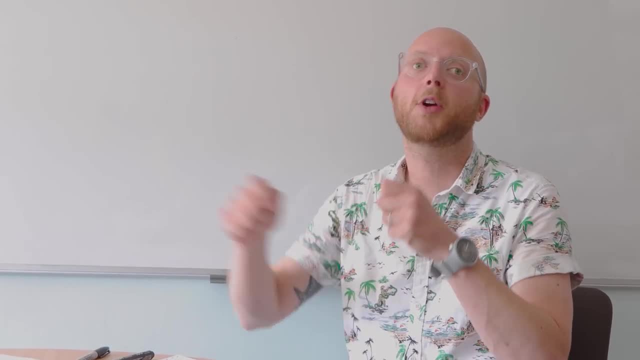 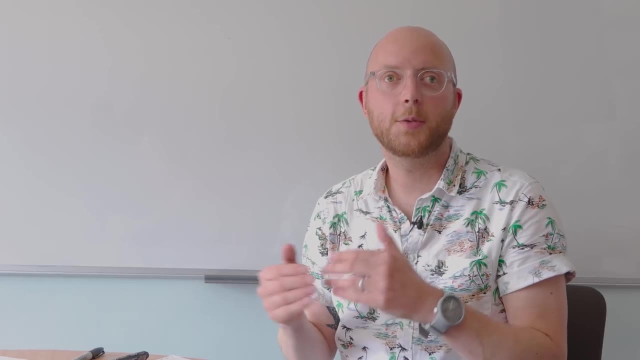 your state to help you make decisions. but, in general, the policy, rather than just being a straight line plan, a sequence of actions, it's going to be a lookup table that says typically, what is the optimal action, so what is the best action to take to achieve a particular specification, so a particular goal. that 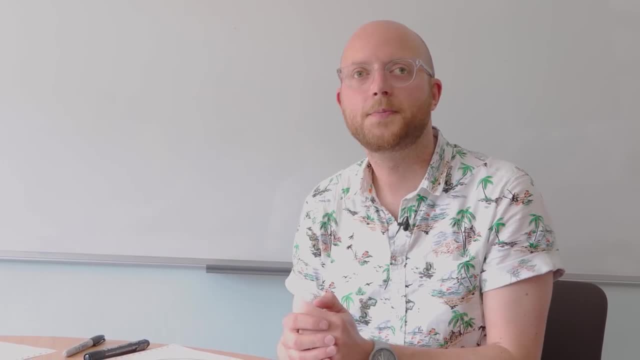 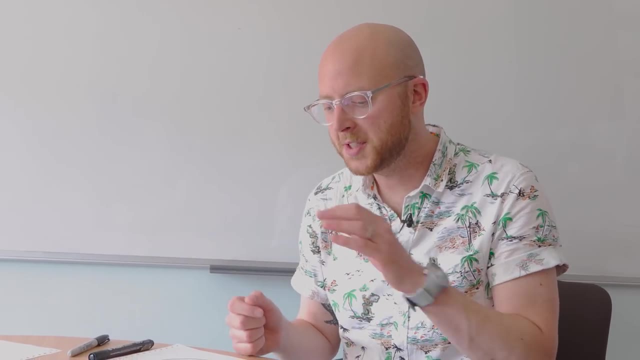 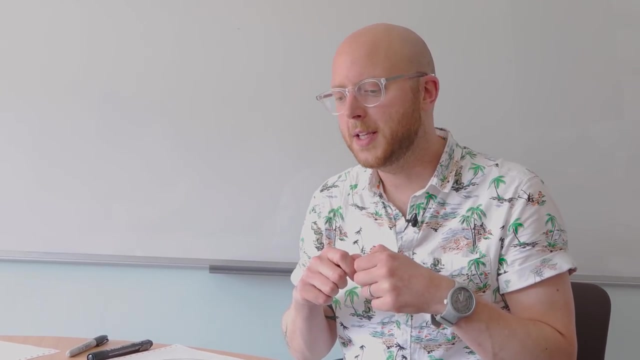 you're trying to reach when you're in this state and you can think of. for mdps there's all sorts of. there's a very rich space of specifications. the most common one for something like this, for a stochastic shortest path problem, is to minimize the expected cost to goal. so the the expected cost is. 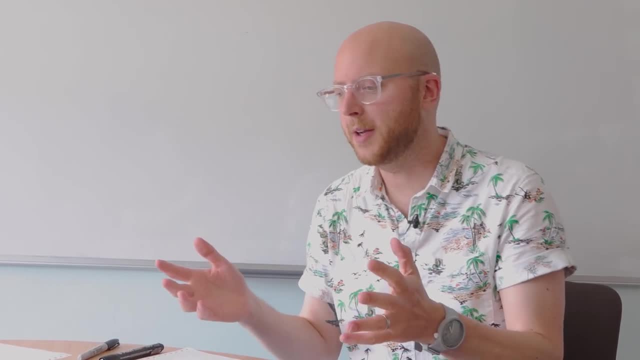 the average cost. so if I get, if I'm going to work, you know, every day for the rest of my life, and I don't have to work every day for the rest of my life and I don't have to work every day for the rest of my life. 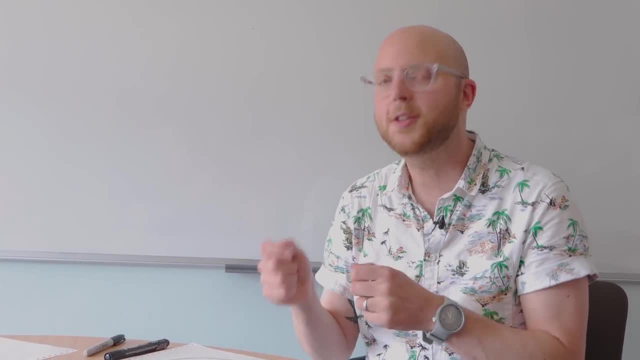 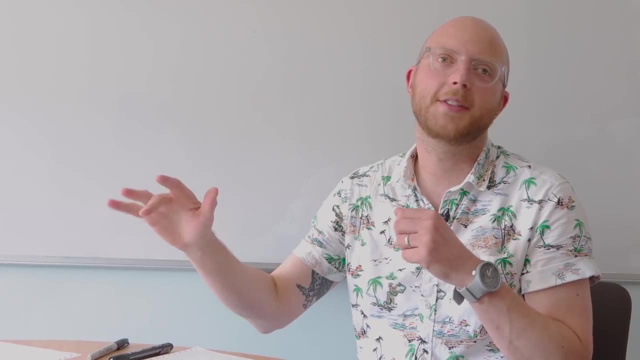 then actually having the expected. so the average cost kind of makes sense, because I get to make this, I get to execute the policy for this, this problem, lots and lots of times- sometimes I do well, sometimes I do badly, but all of that kind of evens out over the time. and so we could, we could think 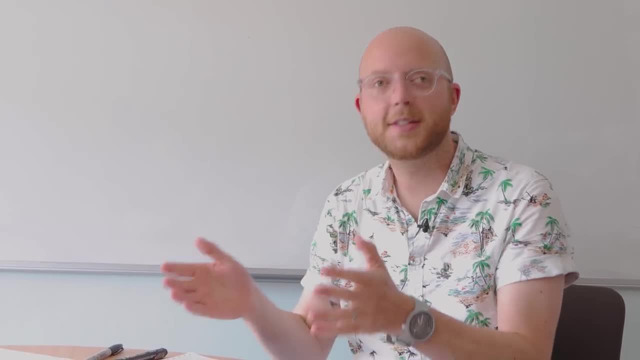 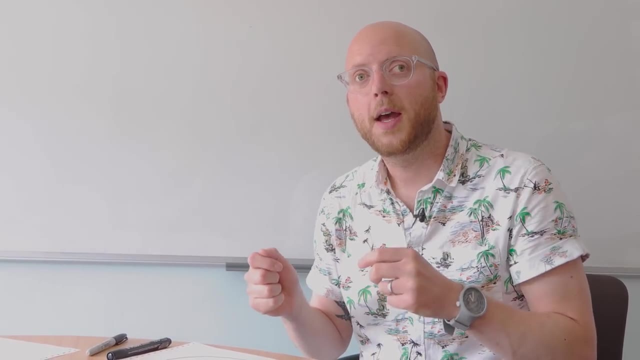 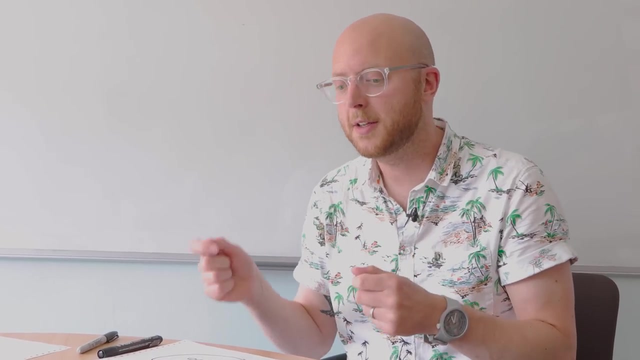 about that to start with, and so my goal is to get to work. my cost is the time, so what I want to do is minimize the cost to get to get to the goal, and that's going to be the cost of the cost, of the expected cost of the whole policy. 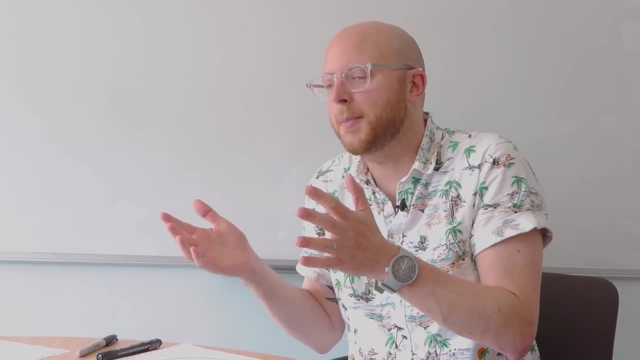 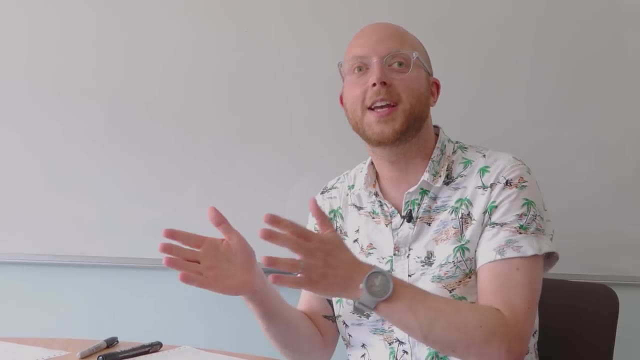 starting from the initial state, which is going to be similar in effect, thinking about the average cost of a path from the start to the end, or the cost of the average path, not the average cost of the path, the other way around, because the paths change because of the probabilities, the way we. 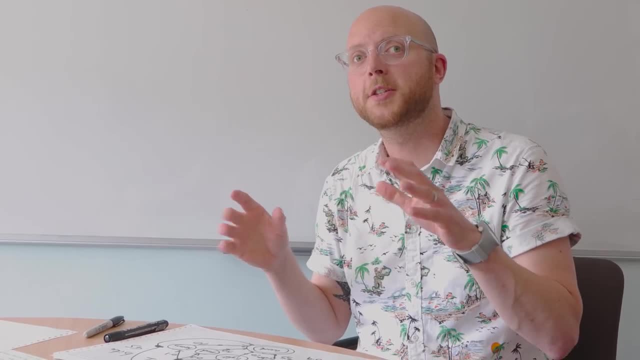 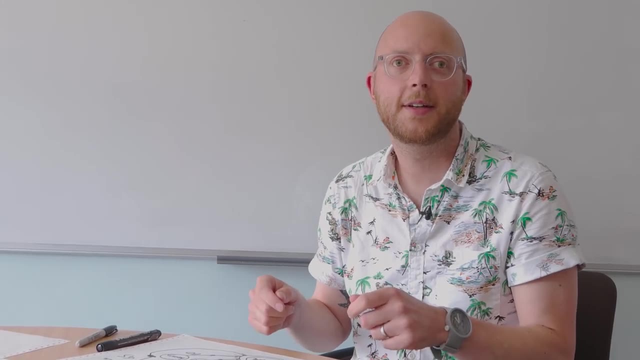 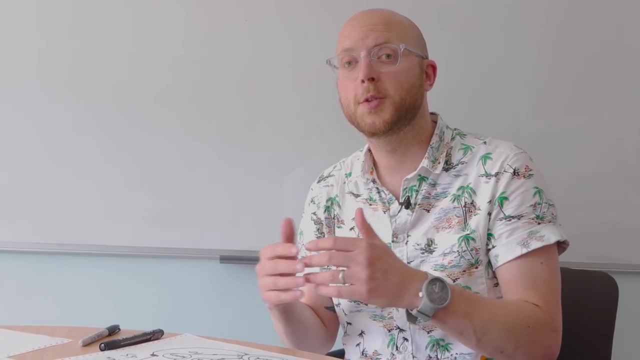 solve this is with something called a bellman equation. so the bellman equation describes how good a particular action choice is. so we need to think about the different action choices available to us in a state. we can evaluate those choices and those we basically pick the best action, which in this 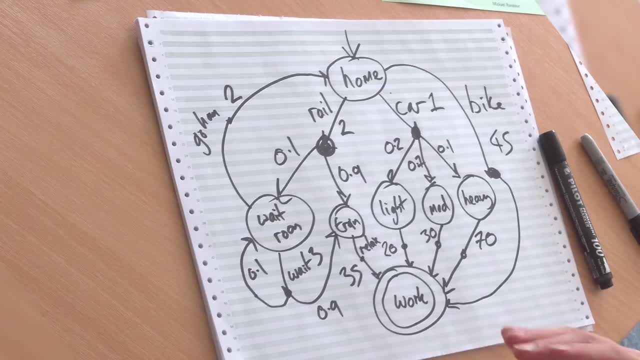 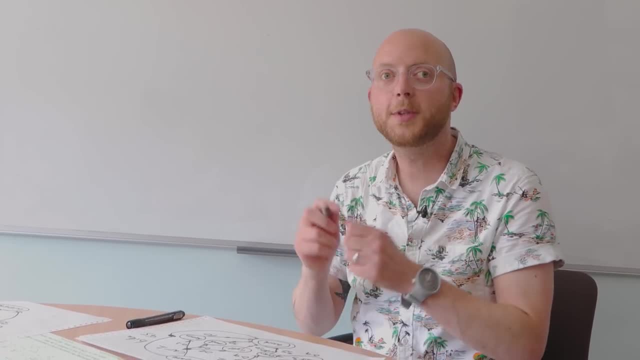 case will be the action with the lowest cost and we put that in the policy. we should also talk about why we can't use things like a star or dykstra. a star and dykstra deal with deterministic problems, so they deal with state transition systems. that might look a little bit like this, but they assume. 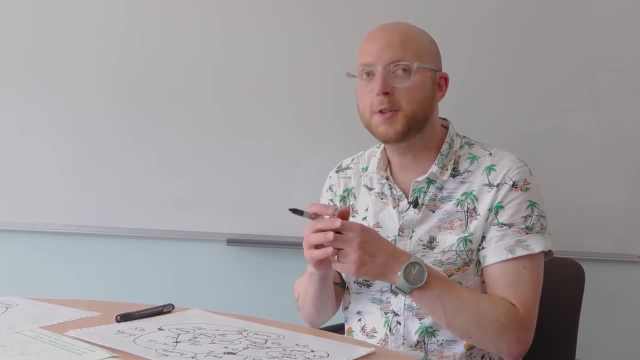 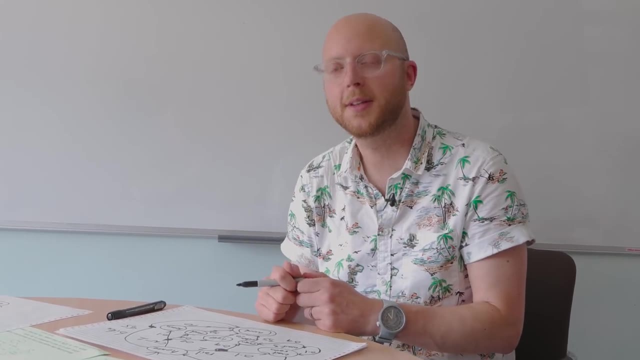 the actions are purely deterministic, so they produce paths from start to finish. there's no probability. there's no probability yet, so they they assume that when they take an action the world changes the way the action behaves. there are kind of analogues for some of these things in the 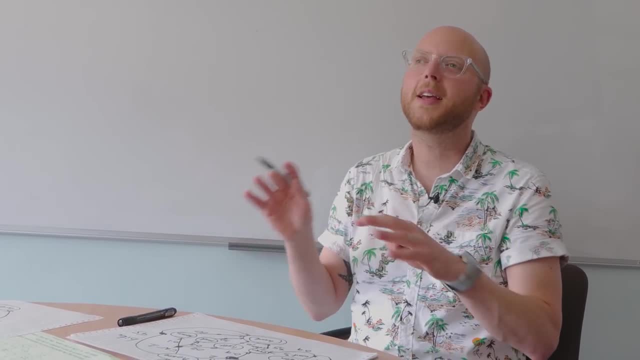 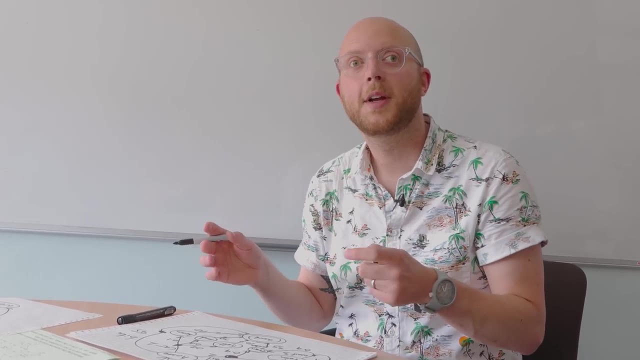 probabilistic world and the the algorithm we'll get to is. it has similarities to the way dykstra's algorithm works and actually a star is a heuristic search algorithm. there are also heuristic search algorithms for markov decision processes, so they're classes of algorithms that fit well. 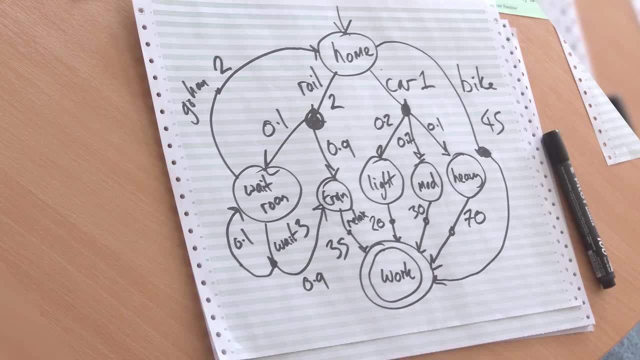 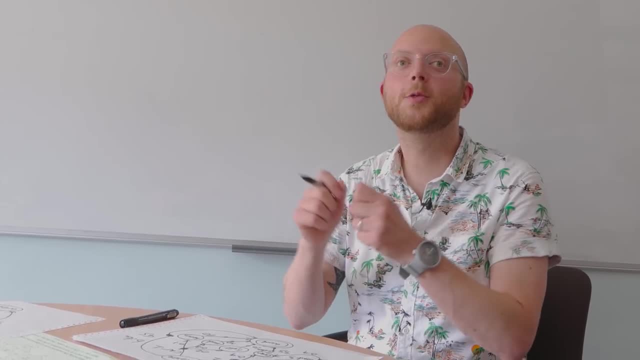 together, and but for this we can't take dykstra or a star and say you know off we go. if you're thinking about just the average cost, then everything gets a lot easier, and we we're. what we're basically going to do is take all the the different act. we're going to multiply the. 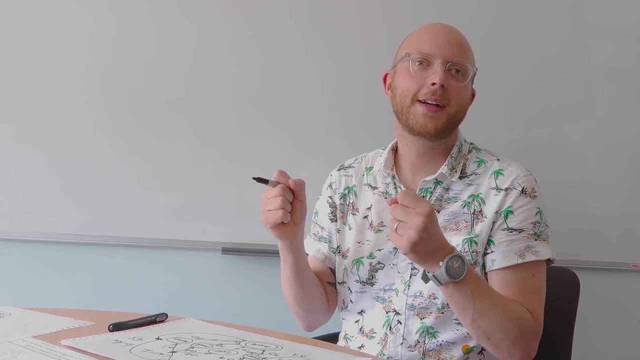 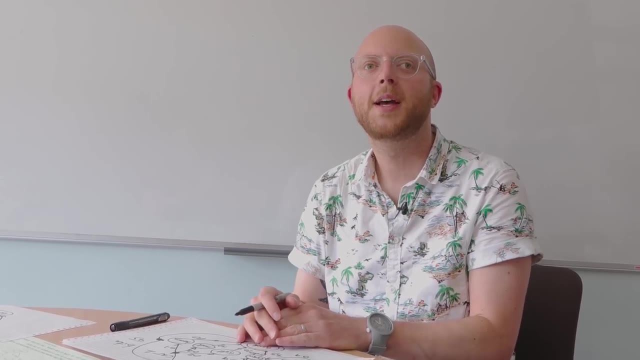 cost by the probability of getting that cost. sum them up and that tells us really how good that action is. so it's just kind of like. it's almost like taking something like a normal shortest path algorithm and collapsing all of the actions into an average action. but we have to do that. 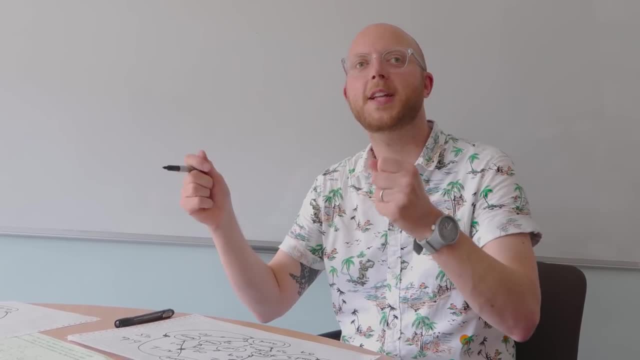 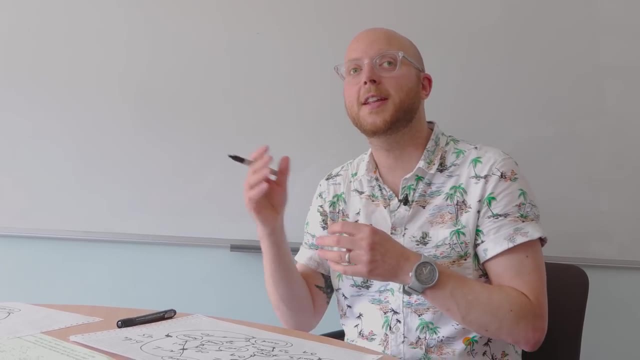 recursively because that each action takes me to another state where i can apply a different. i have to make a different action choice. so we have this recursive problem of my actions are only as good as the states they reach. that's the kind of recursive part. but i also have to 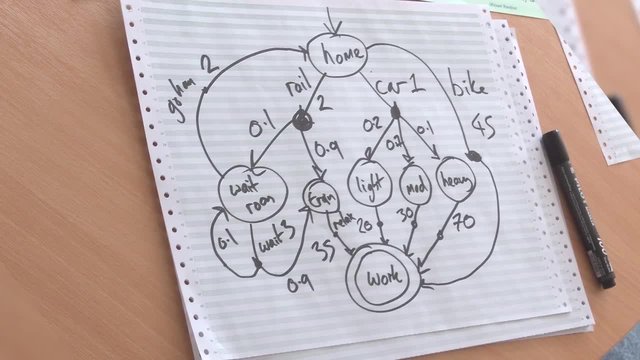 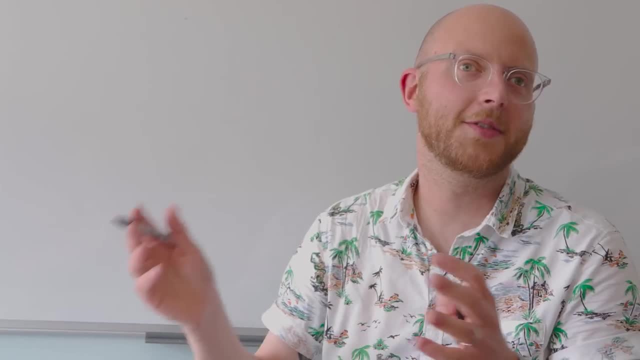 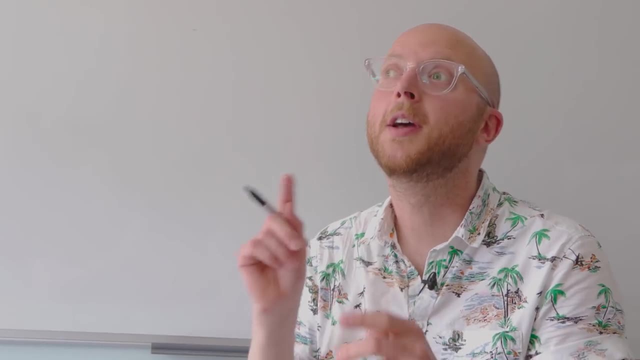 think about the fact that that happens probabilistically, which is where this sort of averaging comes in for the expected cost. we can also think about trying to limit the probability of success or failure or the probability of certain extremes. i think we can talk about that later. um, the algorithms are that much, much harder but but super interesting and actually those are. 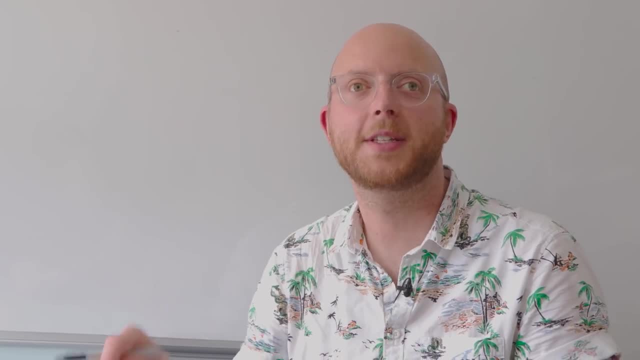 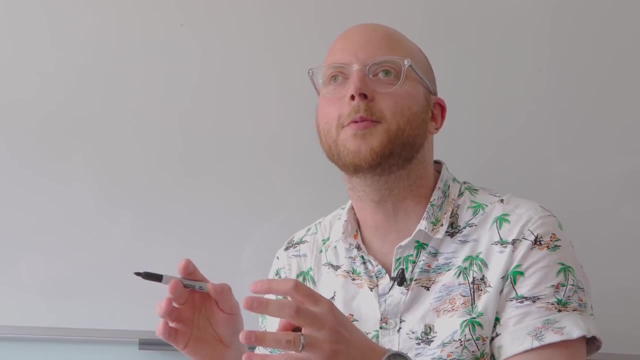 the things you care about when your boss says you have to be here by 10 o'clock for a meeting or your patience runs out if you're an employee at an event of the day, so they can be here by 10 o'clock and you've never been there. 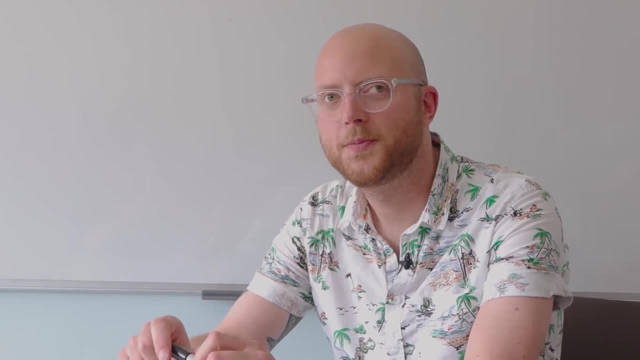 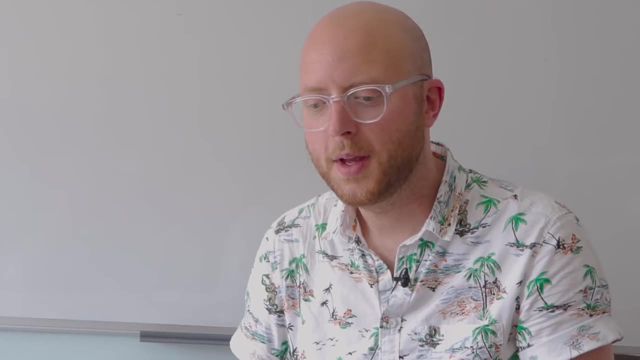 but what happens to those strengths and weaknesses they can really come to an agreement with before they regress? that, uh, yeah, it's a really interesting topic. um, yeah, um yeah, i think the problem with waiting rooms is that you see the performance of a life in a work group. 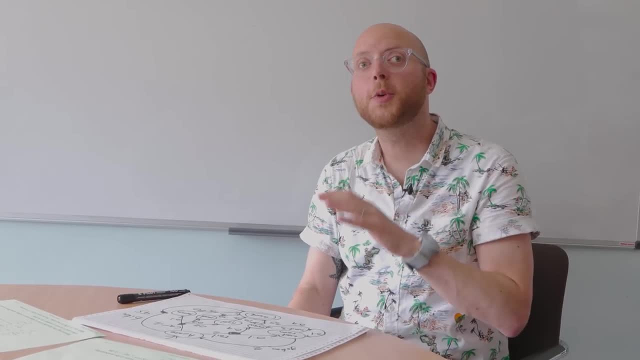 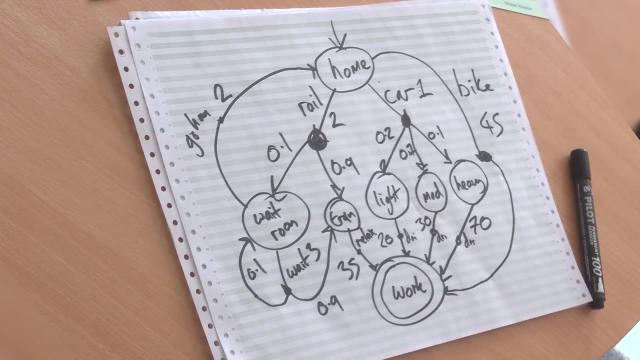 and even if your relationship with it is very good, um, it's like a 30 minute commute is longer than 45 minutes. so real world problems are much. i think real world problems are better captured by those richer specifications. i mean it looks to me like the waiting room is the sort of: is the kicker? choice is car. I think it's something like 33 or 34 minutes, which is faster than bike, which is 45. And I think train comes in somewhere over 35 or over 37 on average. So it's more expensive than. 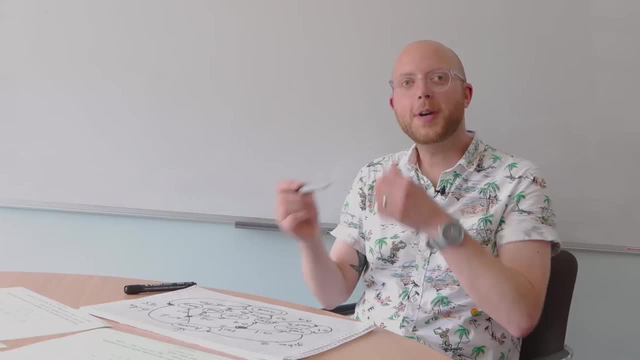 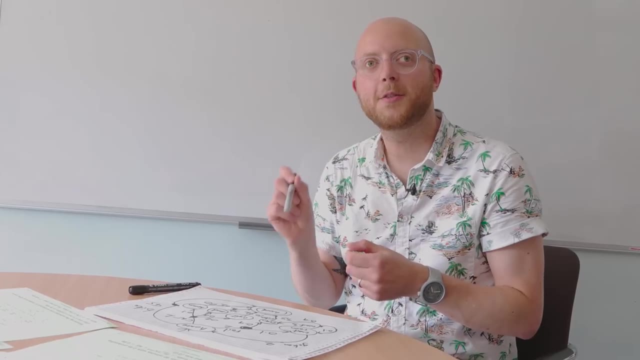 car cheaper than bike. But yeah, the average thing is interesting And this is where these models become fun for robotics and for problem solving, which is by choosing the car. 10% of your journeys take you 71 minutes, which would make you extremely late for work if, in general, you 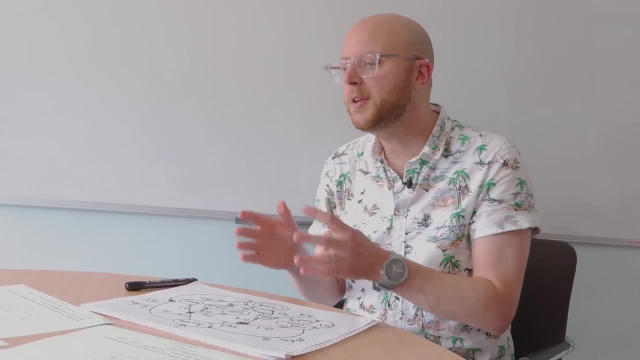 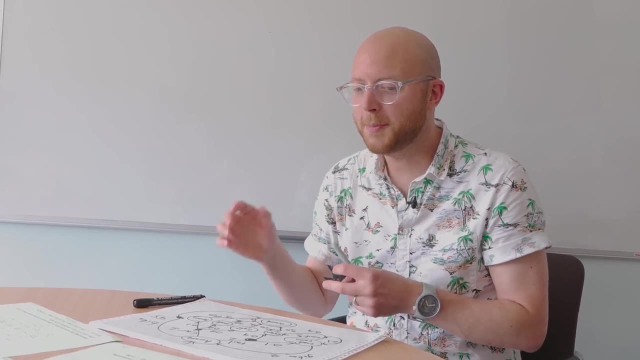 should be taking 30 to 40. So if you only solve for average value, then 10% of the time you're very late, And so what you can think about in these kind of problems is different, what we call either specifications or objective functions. So if you're doing some optimisation, you typically 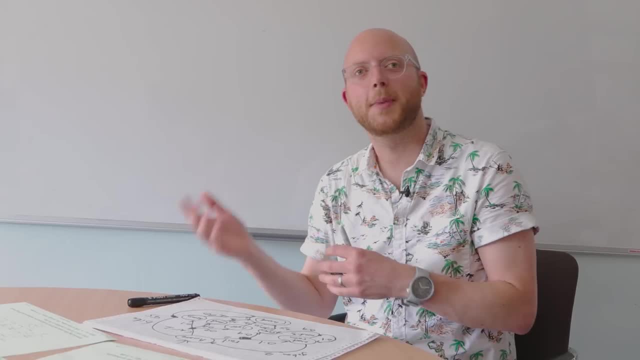 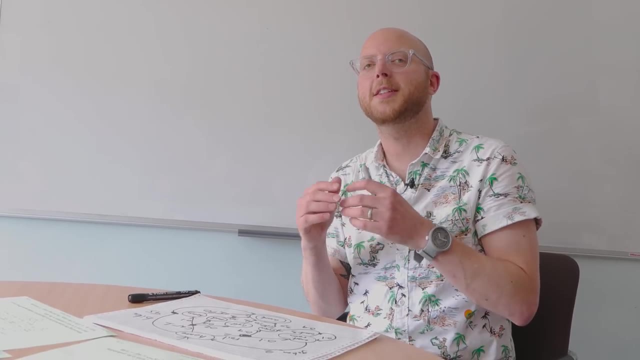 think about the optimisation, the objective function, the thing you're minimising or maximising, And in when we do planning or decision making with these kinds of models, we often phrase it as a specification which is a mixture of the goal you're trying to reach and the constraints you're. 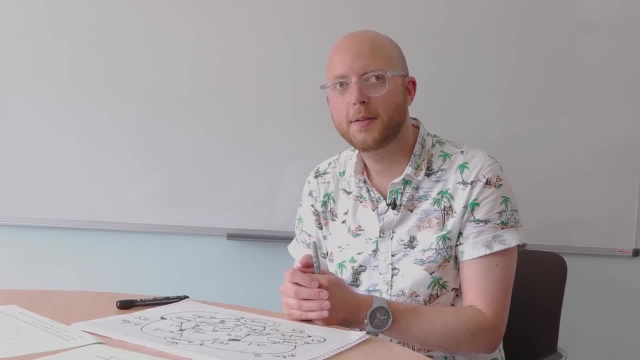 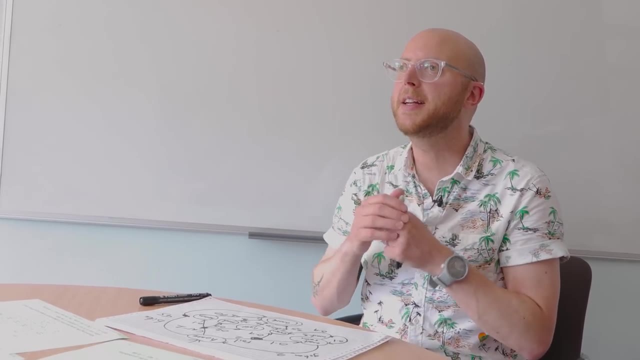 trying to put on it: Yeah. So, for instance, you're trying to do it in the shortest possible time, but it should never be longer than Yeah, that's a perfect example. So, if you try to do it in, if you say it can never be longer than, 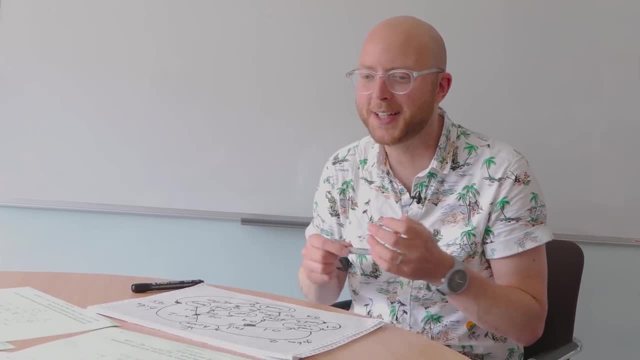 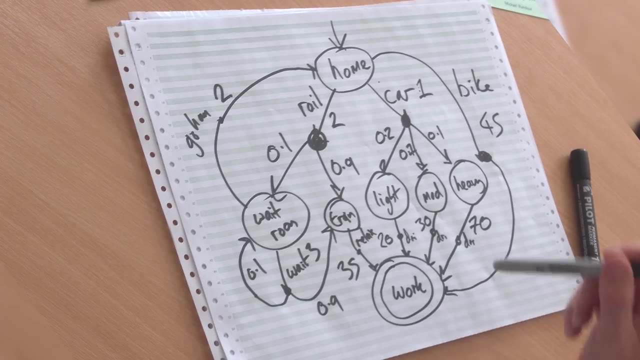 yeah, I'm going to say 60 because the mass. I remember the mass for this. So if you say it for 60, well, you always take the bike Because everything else there's a chance the car takes 70. There is a non-zero probability that the train also takes longer than 60. 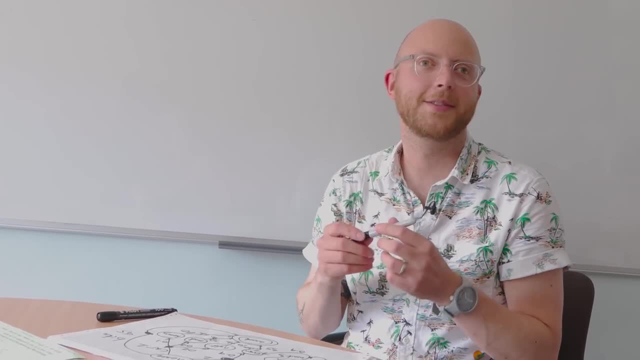 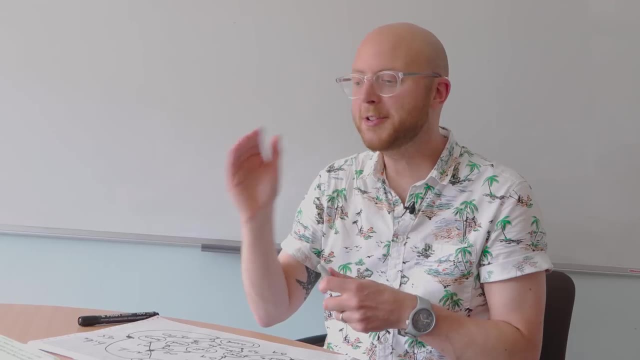 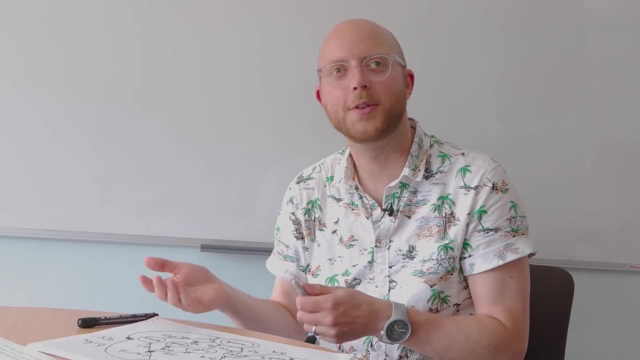 So there is a non-zero probability in the. if you take the train, you're waiting forever, effectively, But the bike is deterministic. but the bike is long, So it's guaranteed to be less than 60, but it's guaranteed to always be 45. So you're always going to be later than you want. 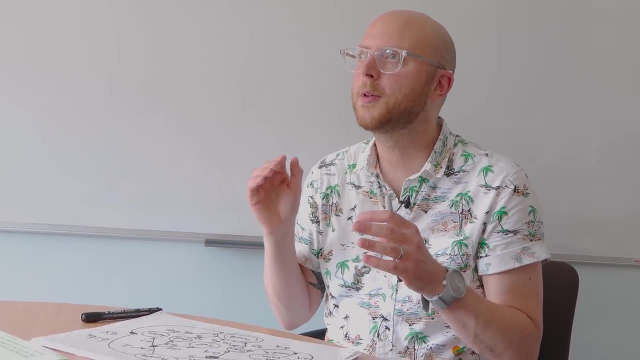 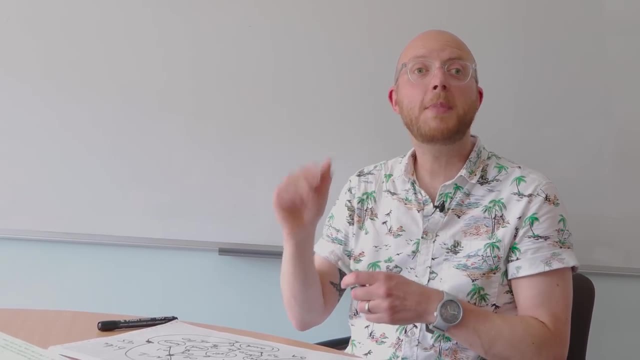 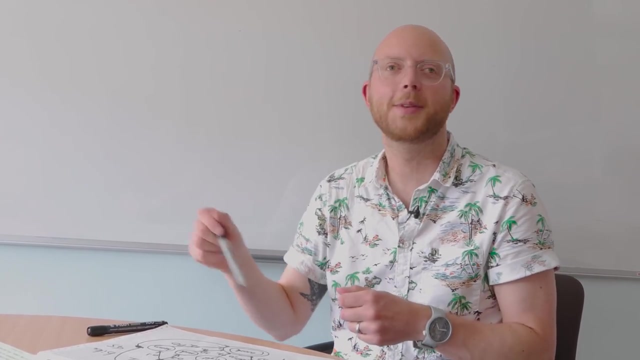 to be, Yeah, The kind of optimal strategy, I think, to get in under 60, guaranteed to get under 60, whilst minimising time, is to go to the train, wait for three cycles and then go home and get the bike So effectively. 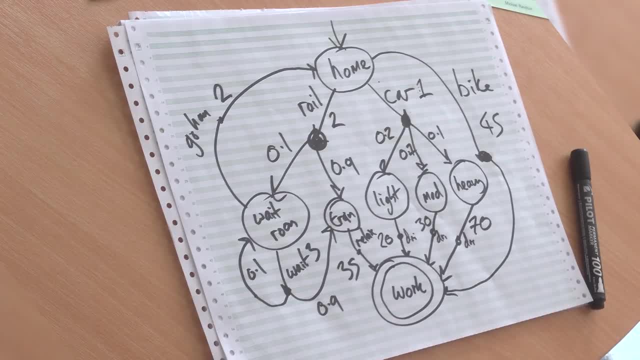 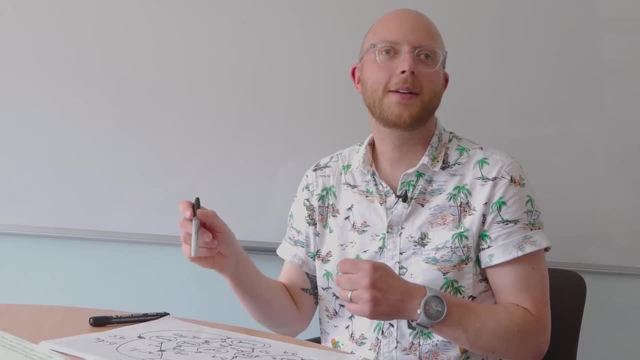 you can think about the chance of getting the train within three cycles, And then, if you go any longer than it's going to take you longer, you'll violate your deadline. So then you go back to get the bike. Yeah, Those kind of solution mechanisms are really. 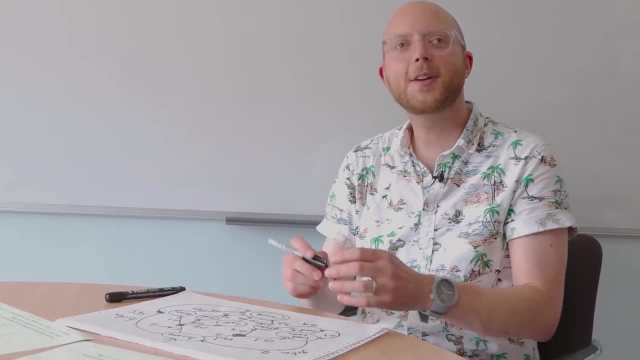 I've actually been in that situation. Yeah, exactly, It happens a lot, particularly kind of post-COVID, where you're like, oh, I could work from home, but I should be there, Oh, the train's late. 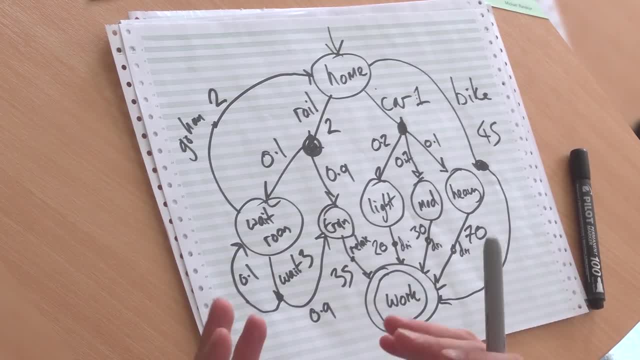 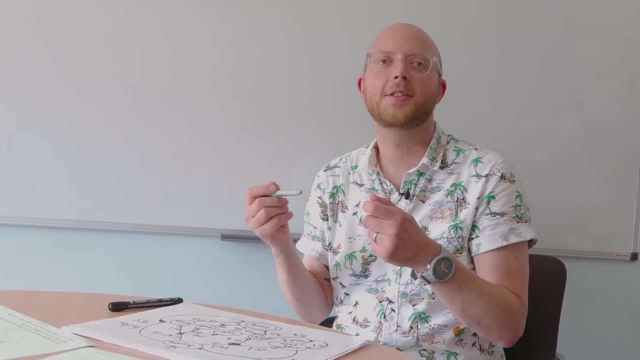 I'm just going to go back and put my pyjamas back on, But you need to think about what we call an augmented state space. You'd put the time that you've waited into the state, and that allows your policy to include actions.